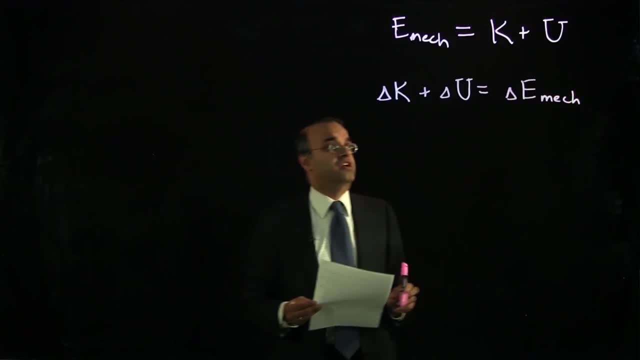 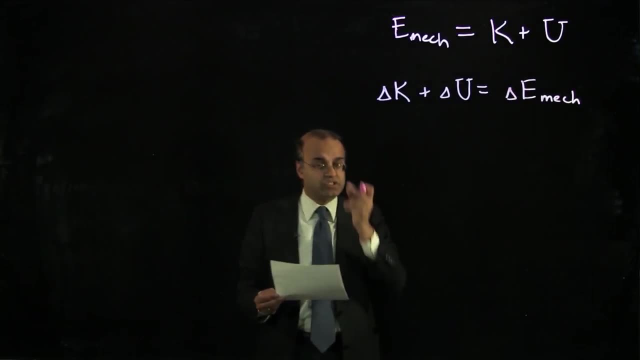 in the potential energy, In the total mechanical energy, And that's just basically the derivative of the equation that I wrote above. And this change in the total mechanical energy will be zero for conservative forces. In addition, we've seen that the change in potential energy is related to the conservative. 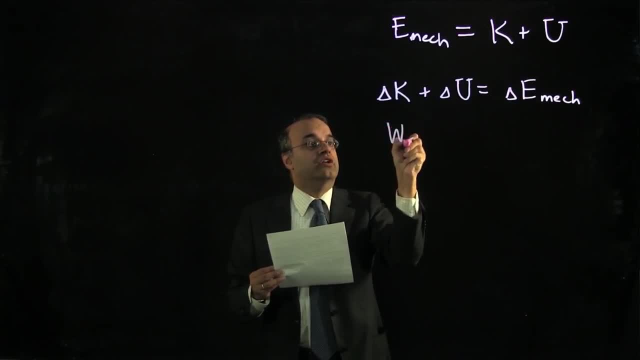 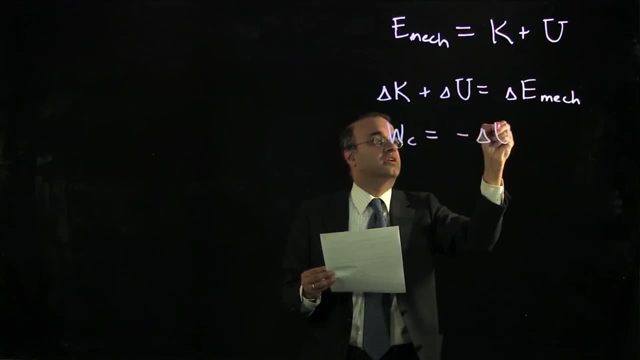 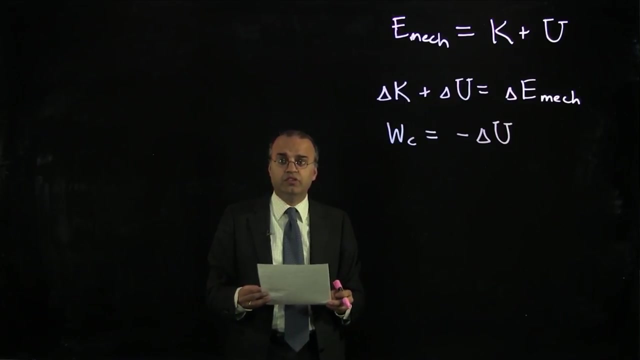 work done in the system so that W sub c the conservative work done is equal to the negative of the change in the potential energy dura sites for cases where negative or positive najin. But we also know that the total work done includes both conservative and non-conservative. 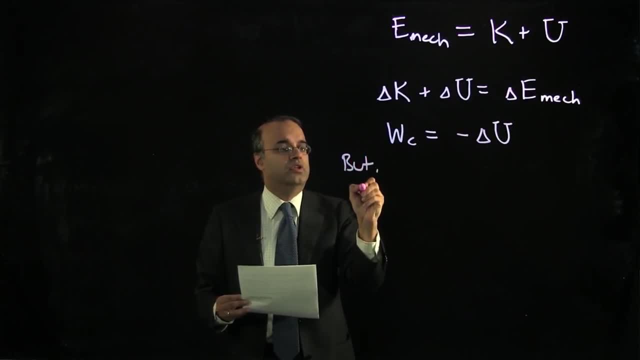 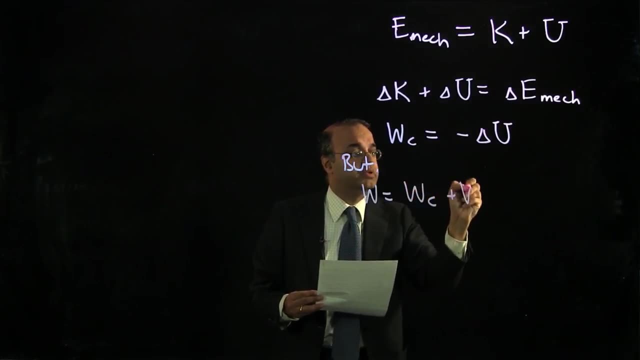 forces, Ecological Yatechnu Or, ahead of time, Conón Perian. So the total work done is equal to the sum of W sub C, the conservative work done plus the non conservative work done, And that that total work is equal to the change in the kinetic. 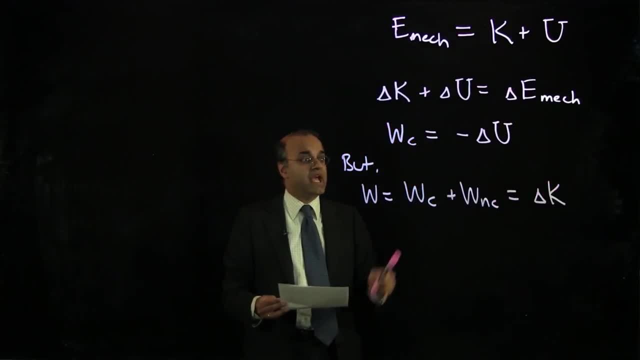 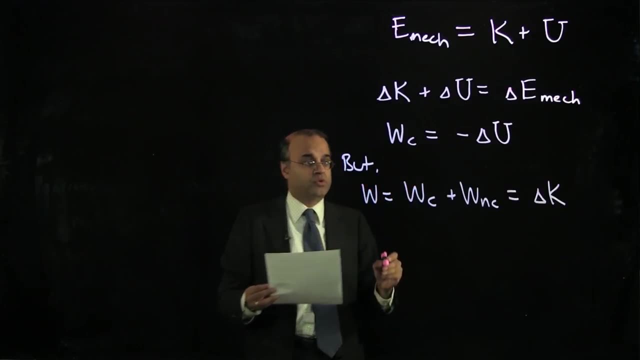 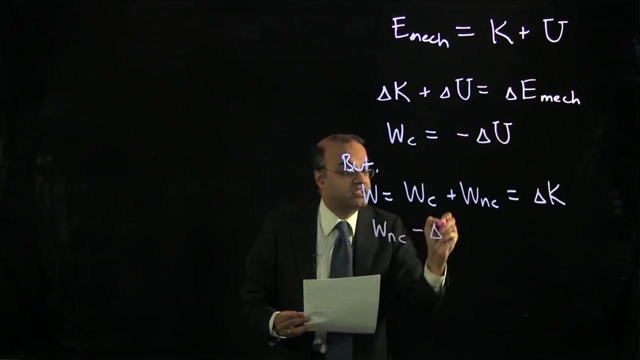 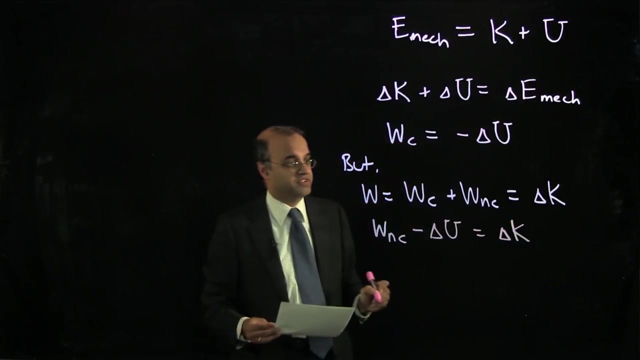 energy functions in kinetic energy. Now I can rewrite that equation by rewriting the conservative work in terms of the potential energy. So I can write this now as the non conservative work minus the change in the potential energy is equal to the change in the kinetic energy. This is again just a restatement of the work. 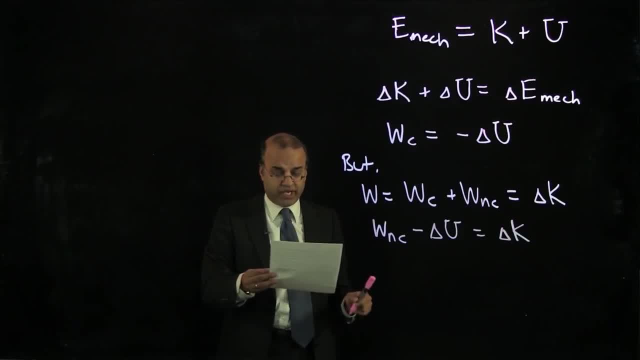 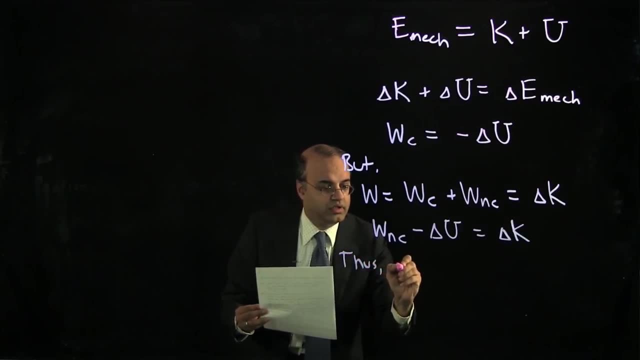 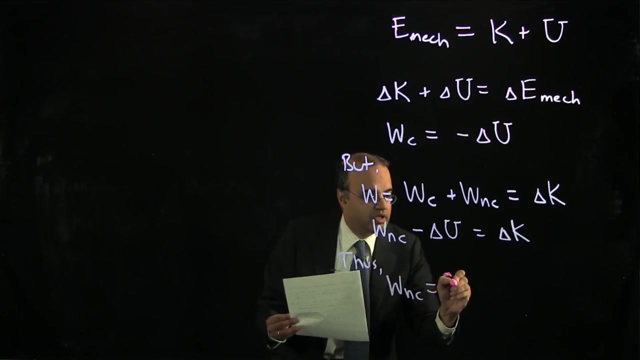 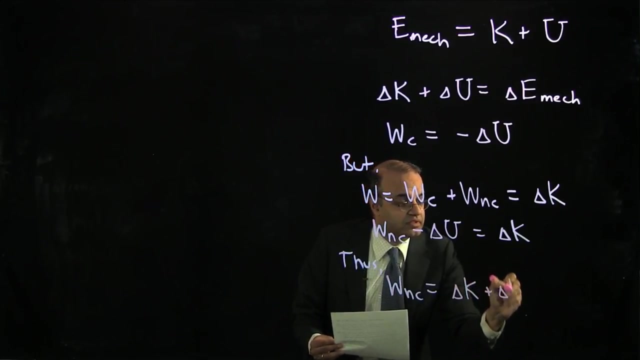 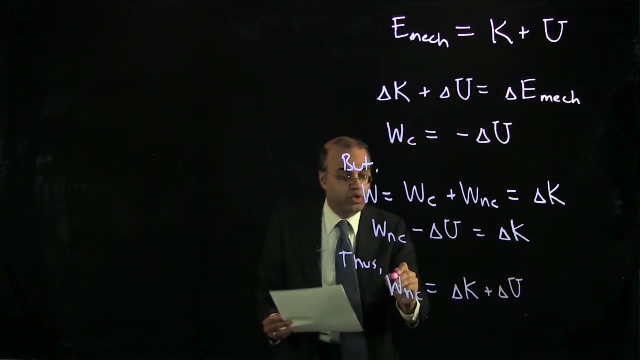 kinetic energy theorem. Now, by rearranging this equation, this means that the non conservative work is equal to delta k, the change in kinetic energy, plus delta u, the change in potential energy. but that's equal to the change in in the total mechanical energy. So the non-conservative work is equal to the change. 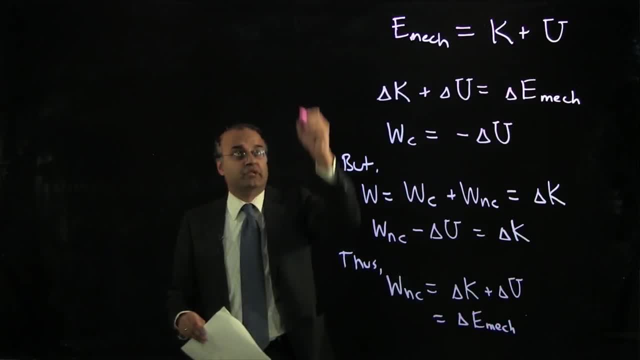 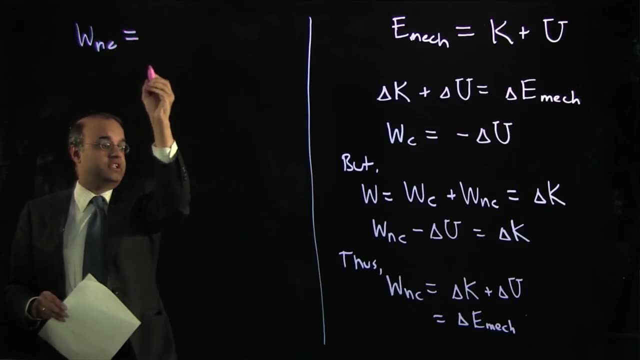 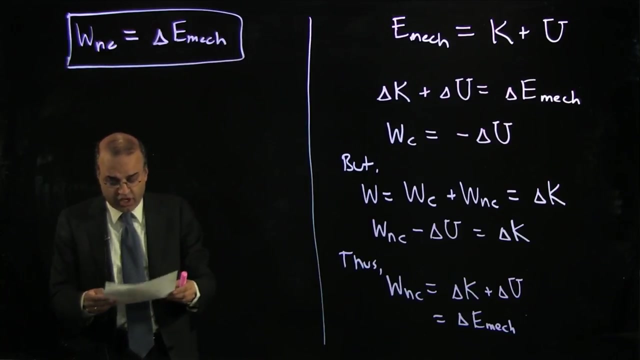 in the total mechanical energy. This is a sufficiently important result that I'm going to write it by itself in a box. So the non-conservative work is equal to the change in the total mechanical energy. So what we've shown here is that the result. 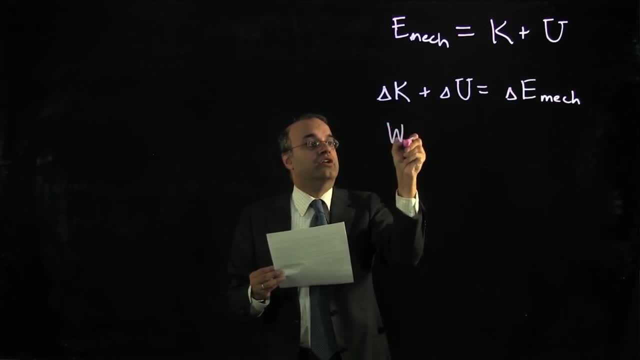 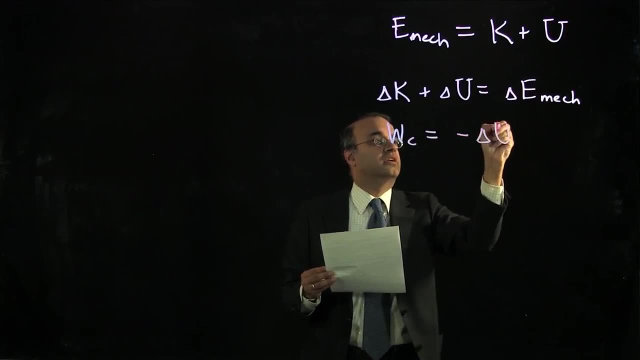 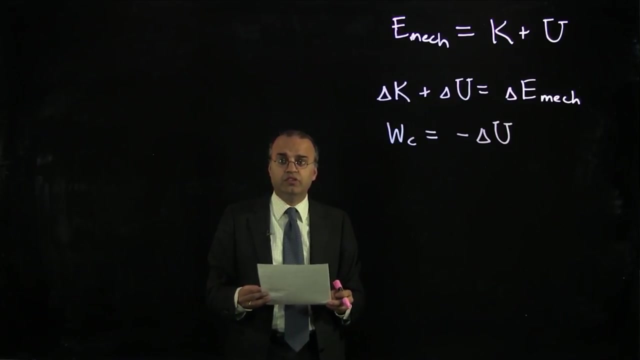 work done in the system, so that W sub c, the conservative work done is equal to the negative of the change in the potential energy. But we also know that the total work done includes both conservative and non-conservative forces, So the total work done is equal to the sum. 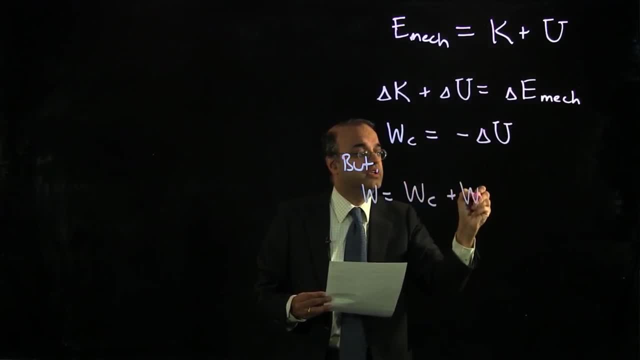 of W sub c, the conservative work done plus the non-conservative work done, And that that total work is equal to the change in the potential energy, The sum of W sub c plus the non-conservative work done, and that that total work is equal to the change in the potential energy. And. 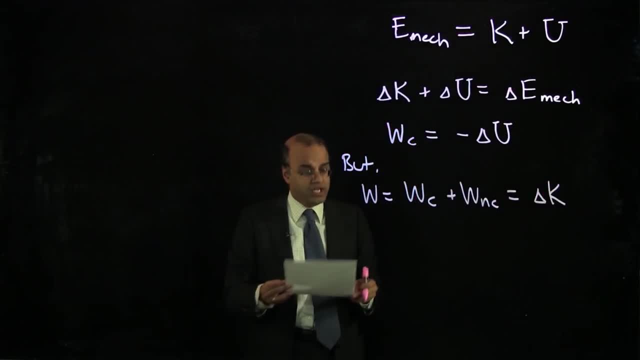 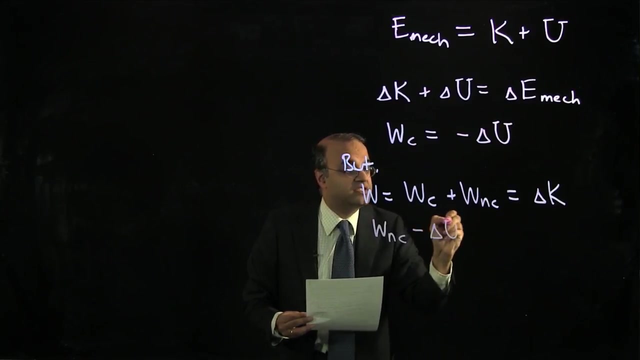 in kinetic energy. Now I can rewrite that equation by rewriting the conservative work in terms of the potential energy. So I can write this now as the non-conservative work minus the change in the potential energy is equal to the change in the kinetic energy. 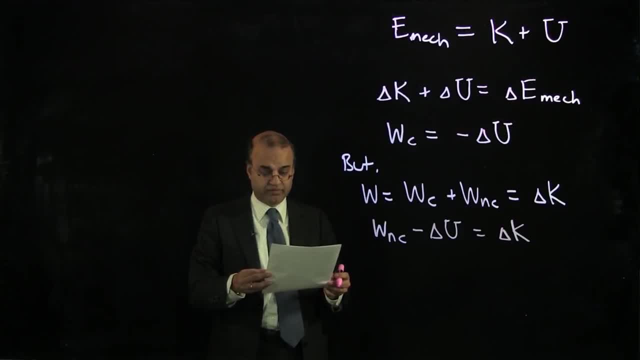 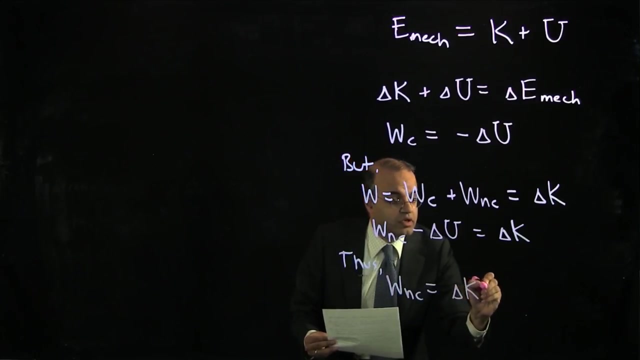 This is again just a restatement of the work kinetic energy theorem. Now, by rearranging this equation, this means that the non-conservative work is equal to delta k, the change in kinetic energy, plus delta u, the change in potential energy. 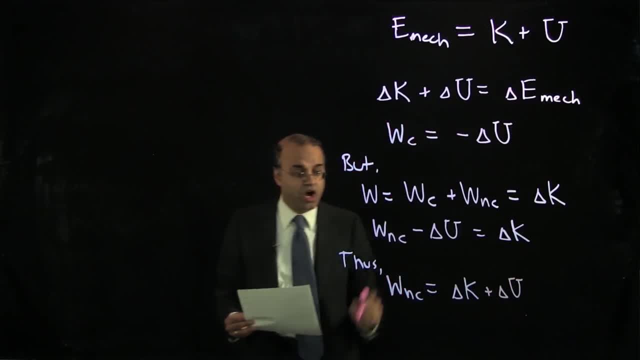 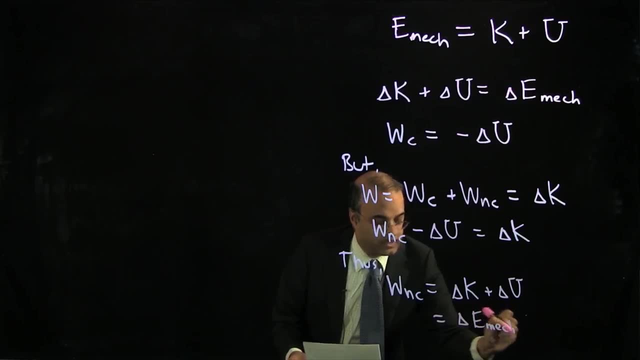 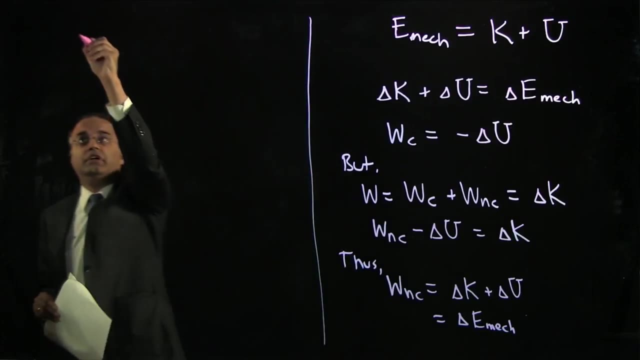 But that's equal to the change in the total mechanical energy. So the non-conservative work- This is the non-conservative work- is equal to the change in the total mechanical energy. This is a sufficiently important result that I'm going to write in by itself in a box. 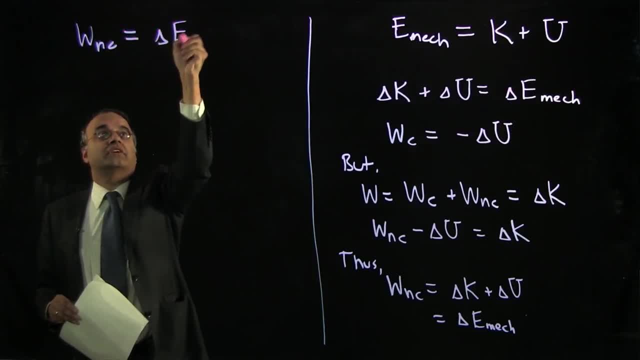 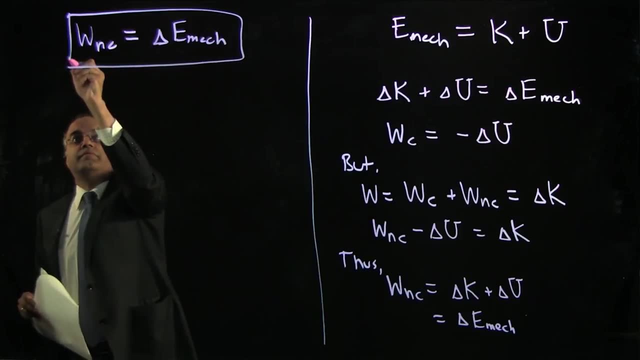 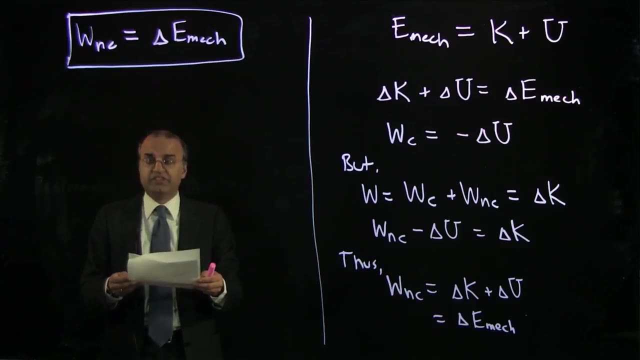 So the non-conservative work is equal to the change in the total mechanical energy. is that the result of any non-conservative work on the system is to change the total mechanical energy of the system? Now, if there is no non-conservative work, 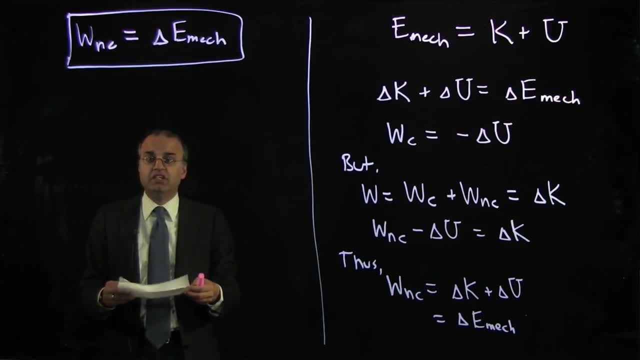 of any non-conservative work on the system is to change the total mechanical energy of the system. Now, if there is no non-conservative work, if the forces acting on the system are all conservative, then the total mechanical energy remains unchanged. Delta E mech is 0, and we say that the total mechanical 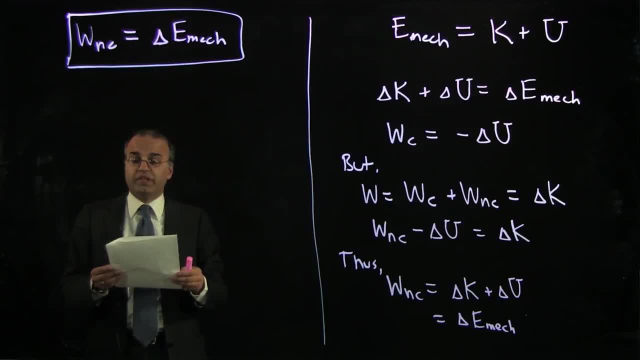 energy is conserved. Now, if there is a non-conservative force? it turns out That, in most cases, the work done by a non-conservative force is negative, resulting in a negative change in the total mechanical energy, In other words, in the removal of total mechanical energy. 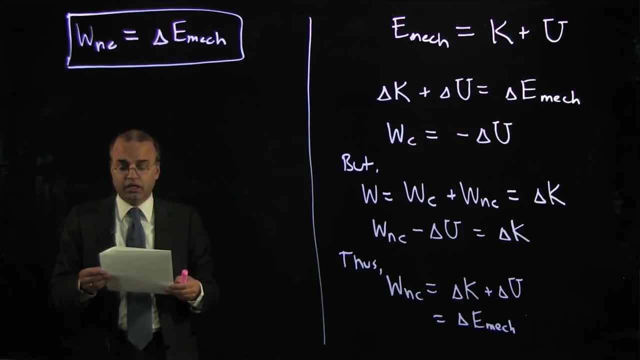 from the system, It's lost from the system. Now we've been talking here only about mechanical energy, which we've defined as the sum of kinetic energy and potential energy, But one can also talk about non-mechanical energy, the most common example of which 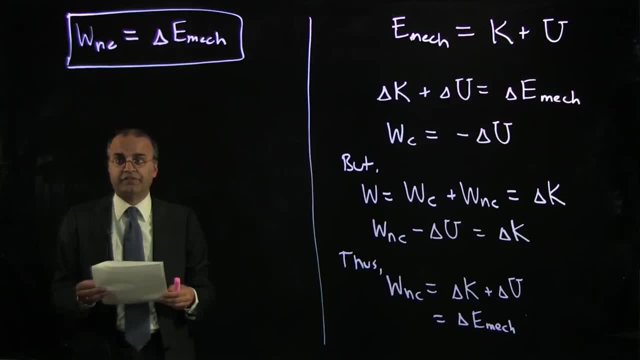 is loosely referred to as heat. As an example, in the case of friction, which is a non-conservative force, we know that the action of friction generates heat. What's happening is that the non-conservative work done by friction is negative and therefore is 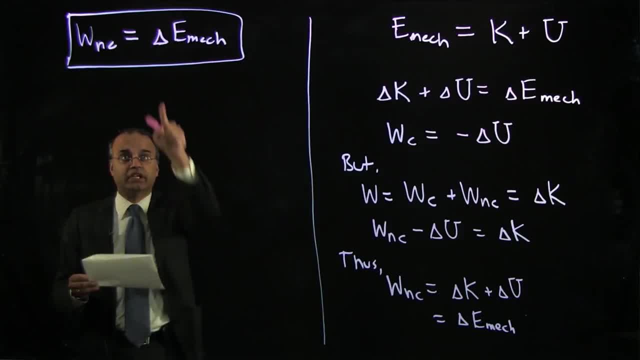 reducing the mechanical energy, the total mechanical energy, according to this expression. But where does that energy go? We said that it's removed from the system in terms of mechanical energy. That's true, But we can think of it As, at the same time, causing an increase. 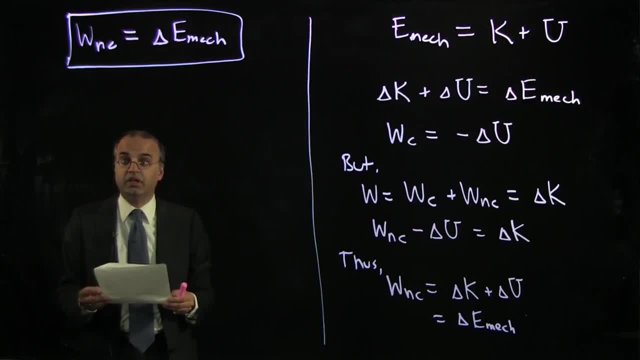 in the non-mechanical energy or the heat energy of the system. So if one were to keep track of both mechanical and non-mechanical energy, then it turns out that the total energy- mechanical and non-mechanical- the total energy of a system. 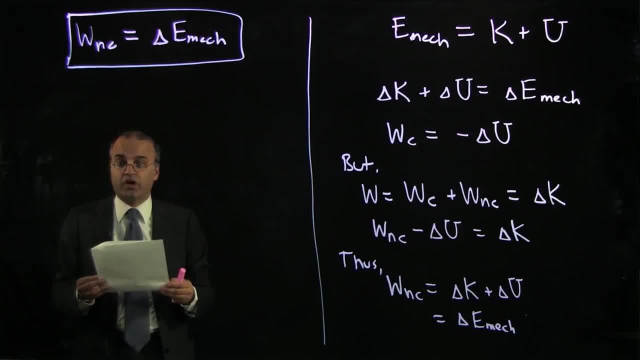 is conserved, even if non-conservative forces are acting. However, it's difficult to recover the non-mechanical energy and change it back into mechanical energy. These non-conservative processes are not reversible. This is a complicated topic and it's the province. 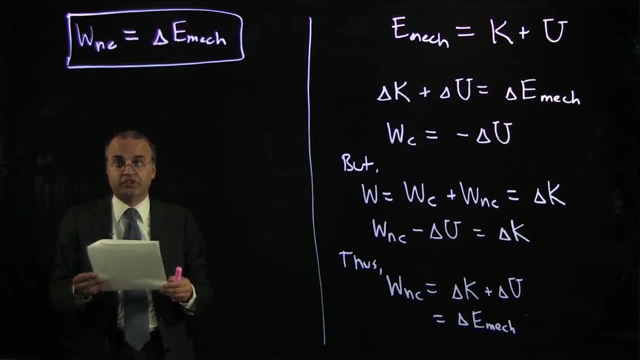 of more advanced courses in thermodynamics or statistical mechanics, which you may encounter later. In this course, we will confine our attention to mechanical energy, the sum of kinetic energy and potential energy, and we'll treat non-conservative force as removing or adding mechanical energy to the system. 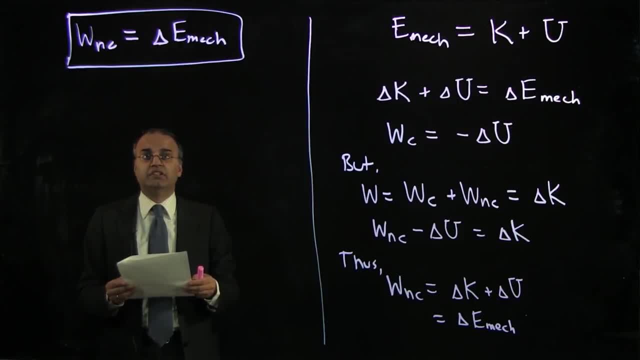 if the forces acting on the system are all conservative, then the total mechanical energy remains unchanged. Delta E mech is 0. And we say that the total mechanical energy is conserved. Now, if there is a non-conservative force, it turns out that in most cases the work 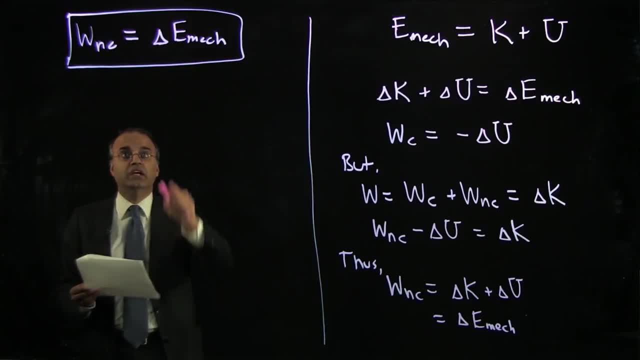 done by a non-conservative force is negative, resulting in a negative change in the total mechanical energy, In other words, in the removal of total mechanical energy from the system. It's lost from the system. Now we've been talking here only about mechanical energy. 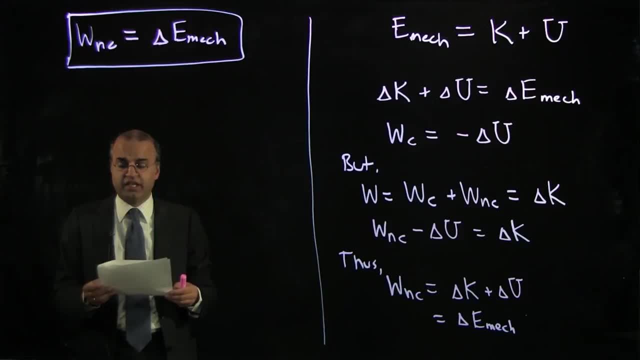 which we've defined as the sum of kinetic energy and potential energy, But one can also talk about non-mechanical energy, the most common example of which is loosely referred to as heat, As an example in the case of friction, which is a non-conservative force. 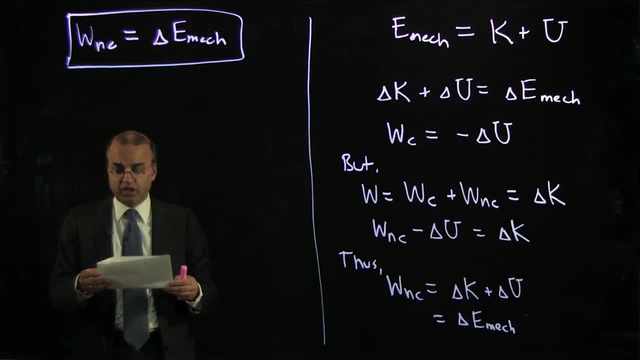 we know that the action of friction generates heat. What's happening is that the non-conservative work done by friction is negative and therefore is reducing the mechanical energy, the total mechanical energy, according to this expression. But where does that energy go? 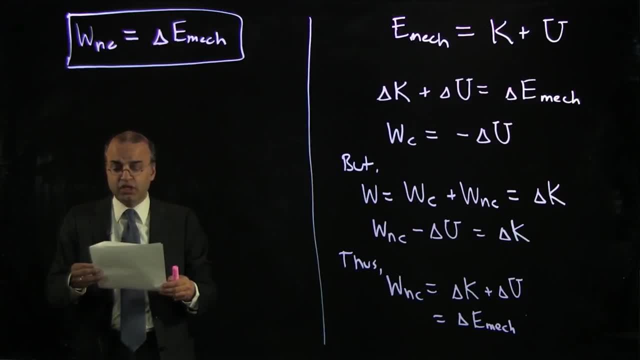 We said that it's removed from the system in terms of mechanical energy. That's true, But we can think of it as, at the same time, causing an increase in the non-mechanical energy, or the heat energy of the system. 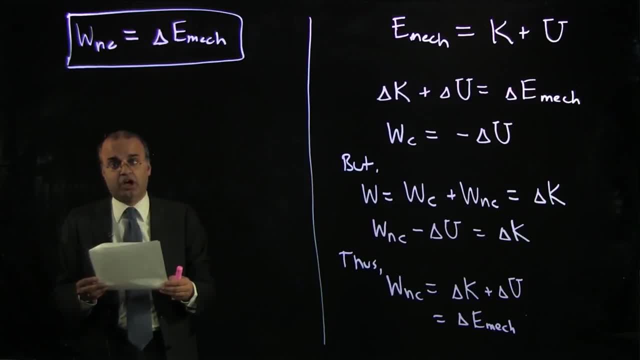 So if one were to keep track of both mechanical and non-mechanical energy, then it turns out that the total energy- mechanical and non-mechanical- the total energy of a system is conserved even if non-conservative forces are acting. 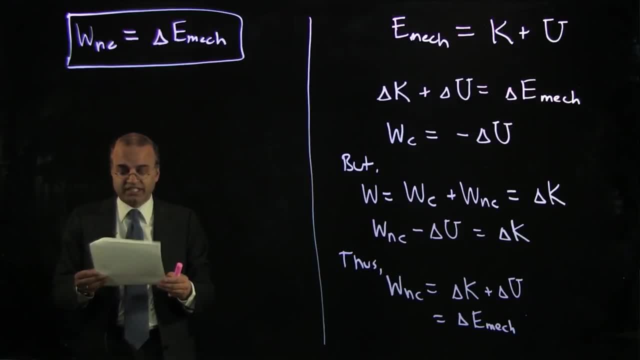 However, it's difficult to recover the non-mechanical energy and change it back into mechanical energy. These non-conservative forces, These non-conservative processes are not reversible. This is a complicated topic and it's the province of more advanced courses in thermodynamics. 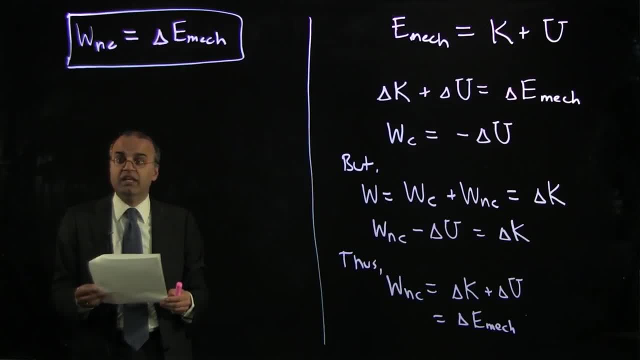 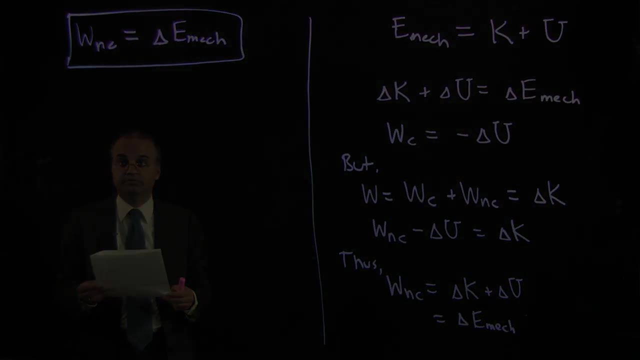 or statistical mechanics which you may encounter later. In this course, we will confine our attention to mechanical energy- the sum of kinetic energy and potential energy- and we'll treat non-conservative force as removing or adding mechanical energy to the system. Subtitles by the Amaraorg community.